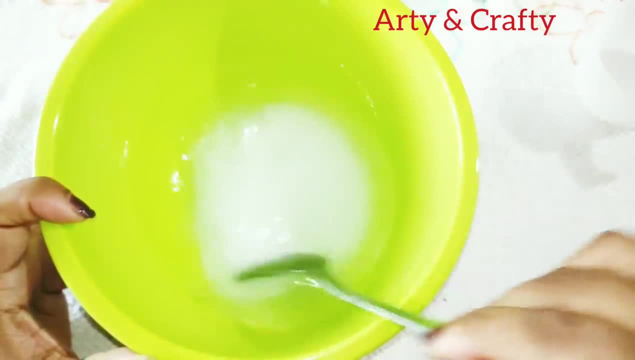 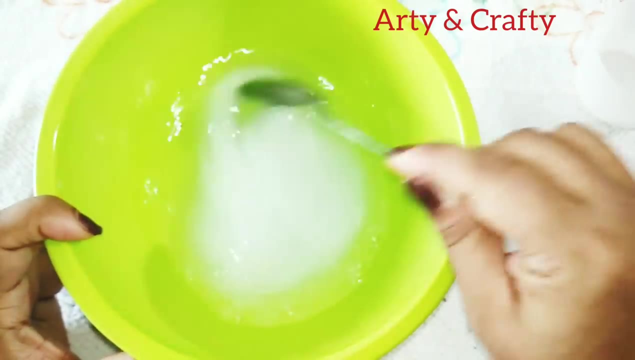 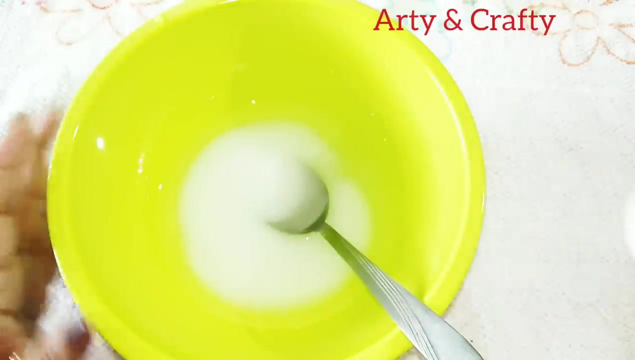 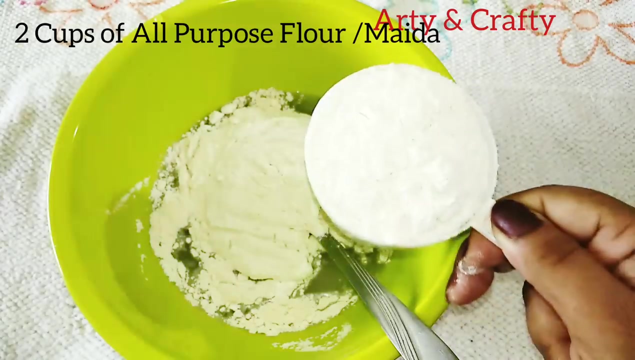 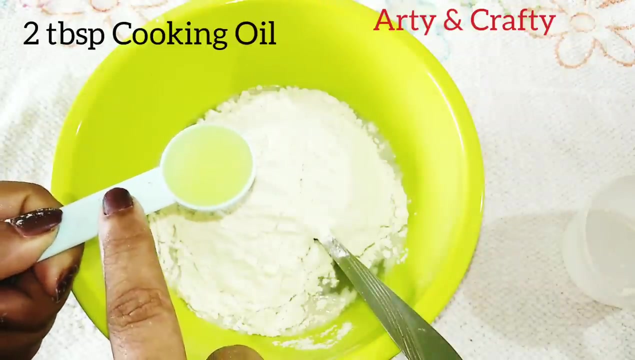 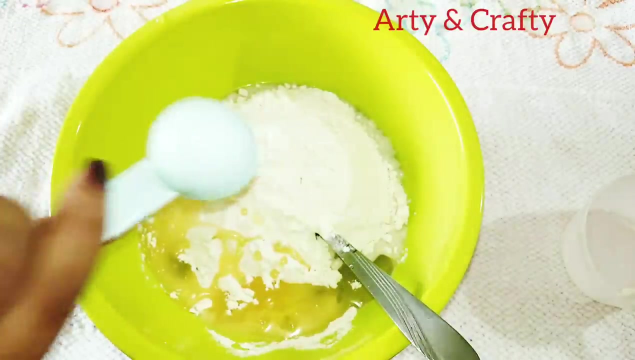 Just keep on stirring till the salt gets dissolved in the water. It will not completely dissolve, but try to dissolve as much as possible. Now we will add 2 cups of all purpose flour, that is maida. Now add 2 tablespoons of cooking oil. Now we will knead it. 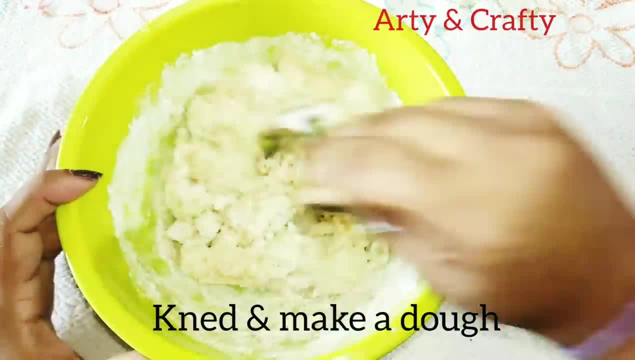 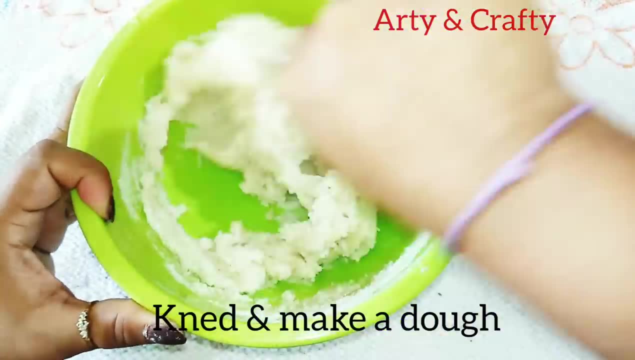 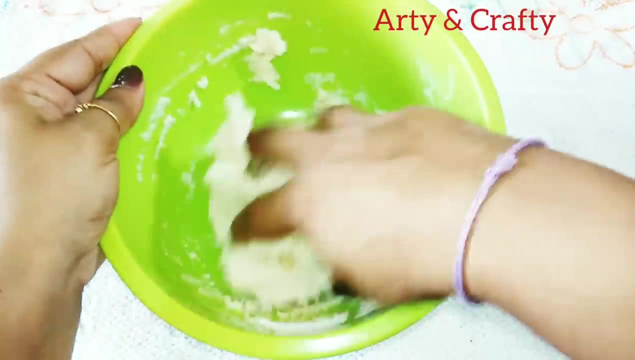 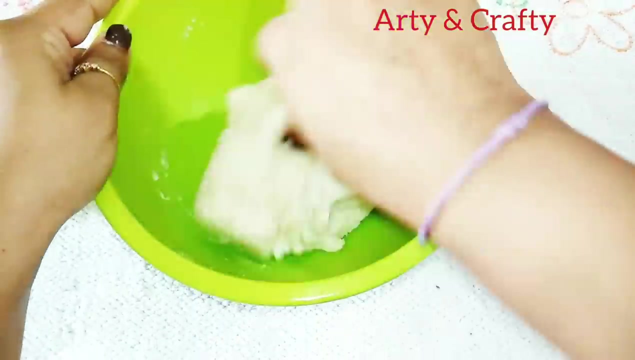 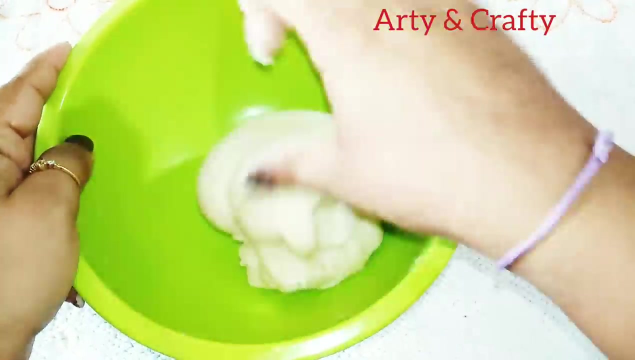 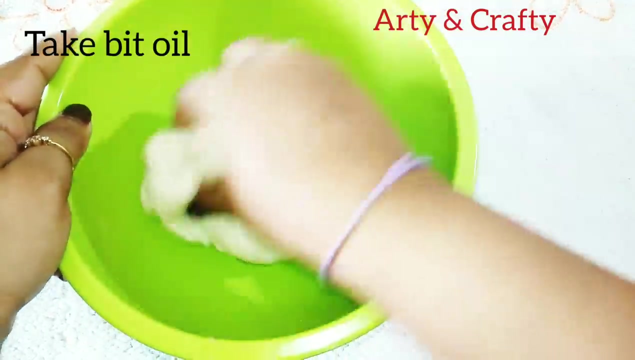 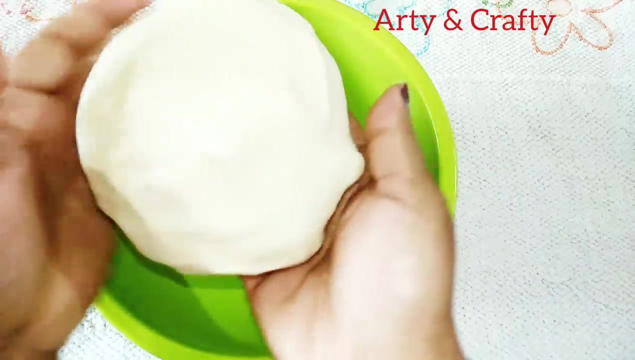 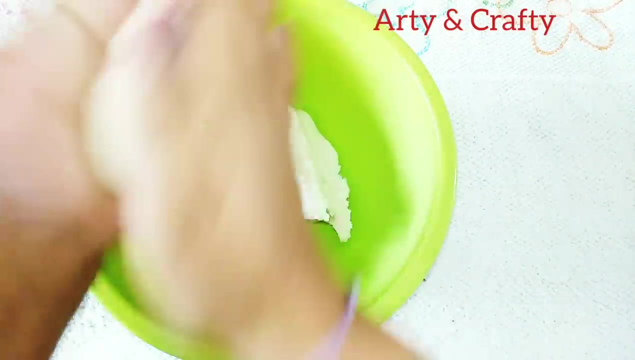 Knead until it should be smooth. Continue kneading for 10 minutes by mixing at the time of drying, so that it does not dry at all. See, the dough is ready. now I will show you. just take a little amount and do this, see. 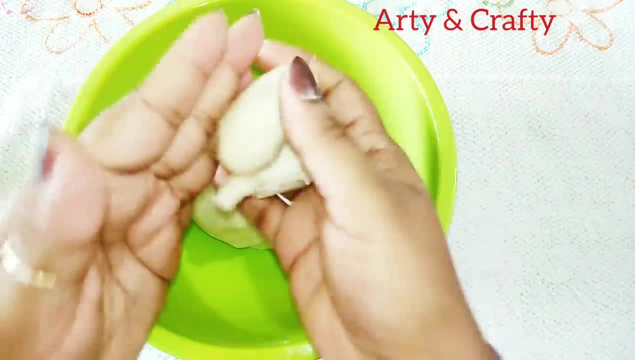 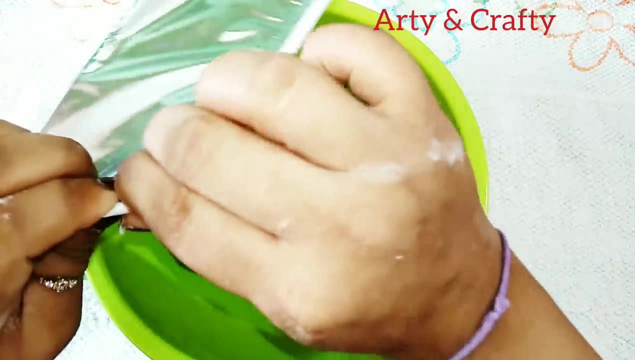 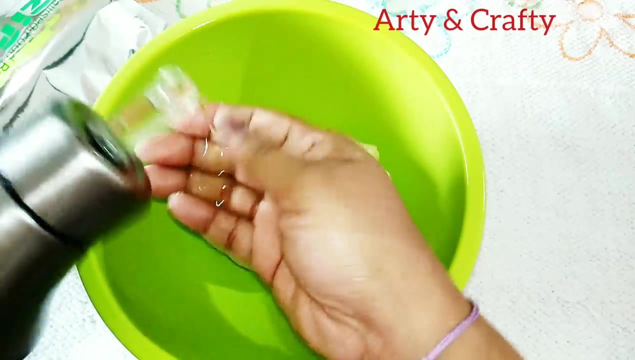 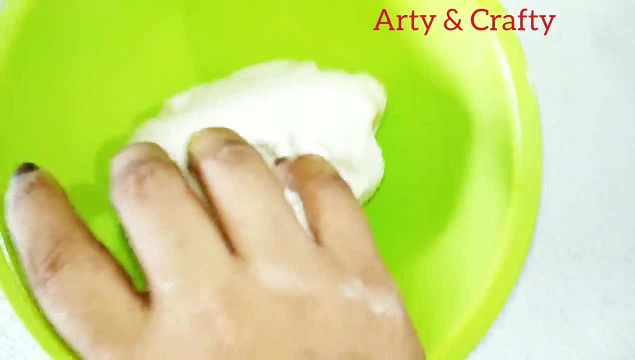 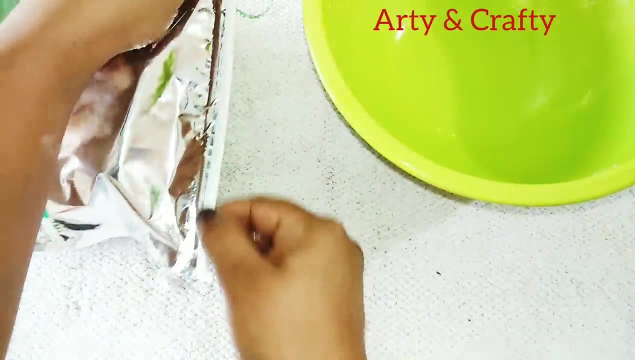 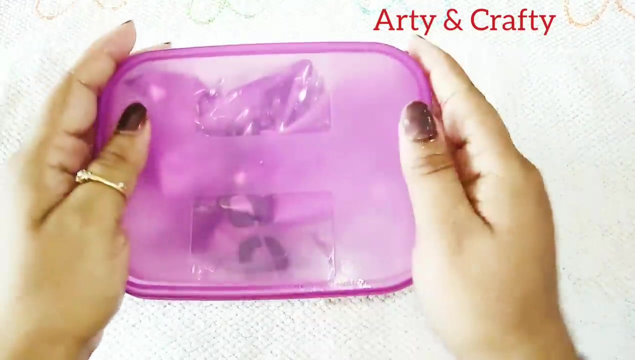 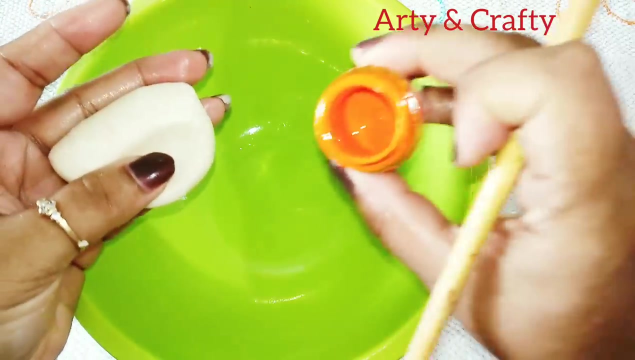 this teardrop forms. this means the clay is perfect. so now peel it properly and take a zip lock bag, just apply oil on it And then you can store it in a container- air tight container. and this you can store it in freeze for up to one month. some clay- I will show you how to color it. I am taking 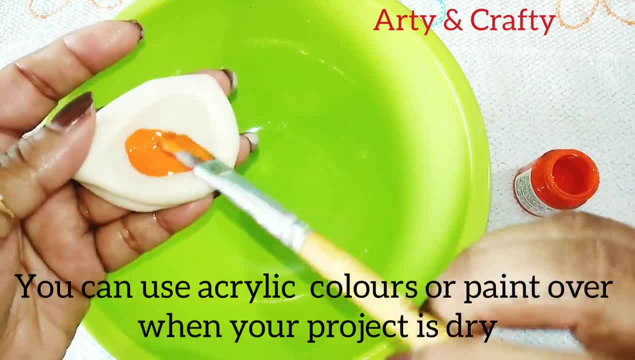 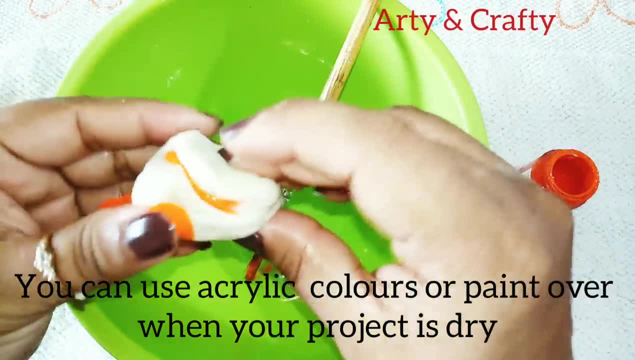 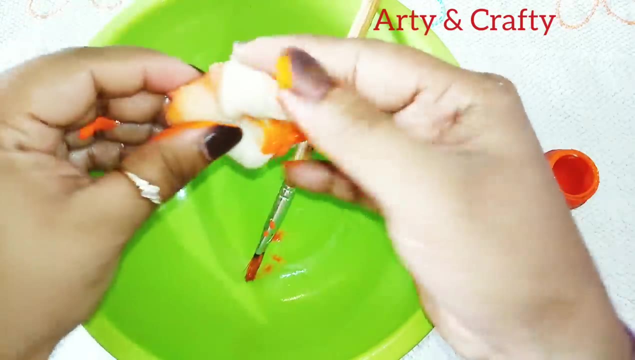 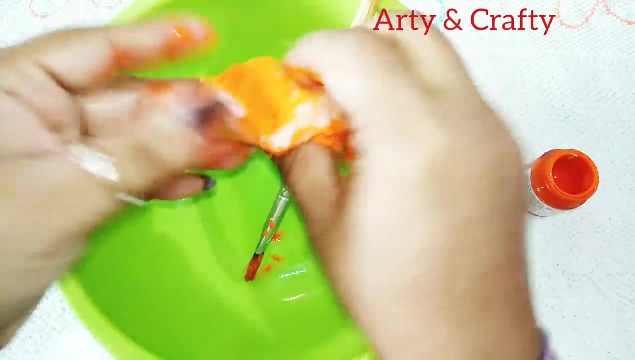 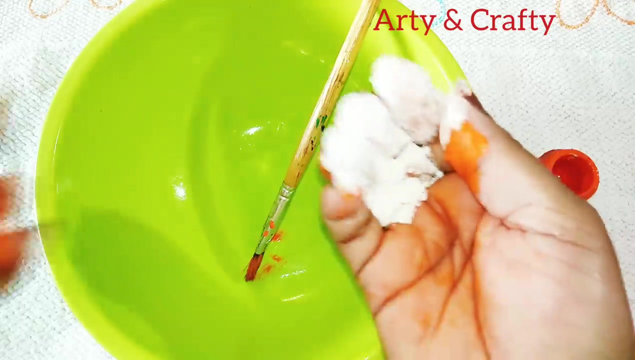 this acrylic color. you can add in the color this manner: just mix it. you can also use it. you can always add the floor when you think the consistency is sticky. so this is acrylic colors. I am adding some floor to it. you can always keep on adding floor, or